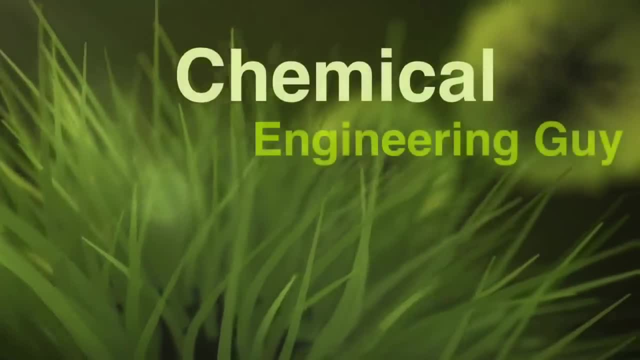 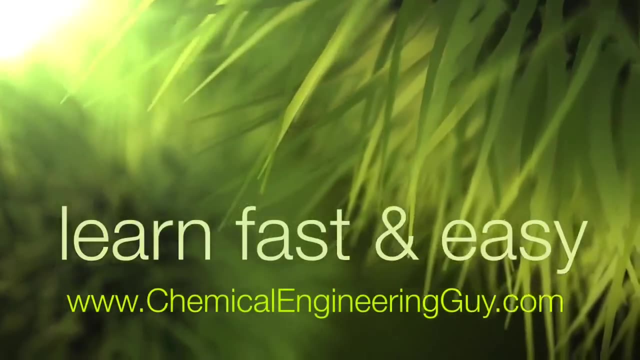 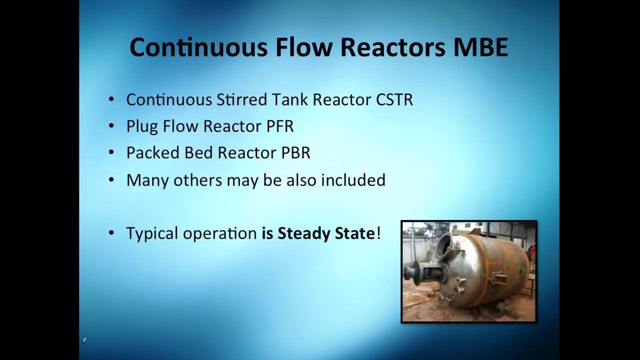 what's up, guys? let's continue with this. continuous flow reactors. we're going to apply the molar ball balance equations. we're going to see three, which is the CSTR, continuous steered tank reactor, plug flow reactor, which is PFR, and the packed bed reactor, which is PBR. you can, you could also do many others, but these. 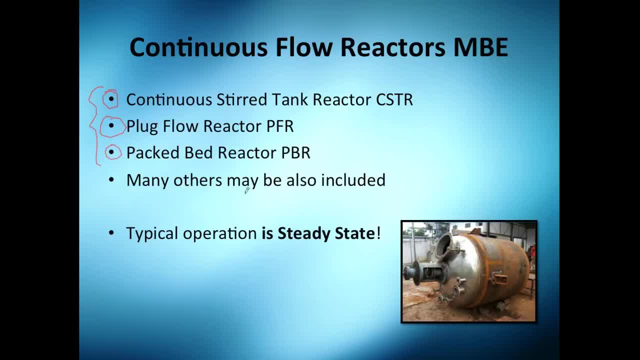 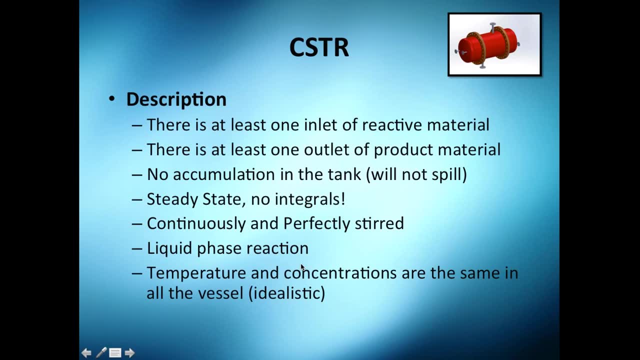 are the typical ones and we're going to use now. this is typically a steady state operation because it's a continuous flow, so there's no accumulation by definition. so let me continue with the CSTR, the continuous steered tank reactor. description: there is at least one inlet of reactive material and there is at 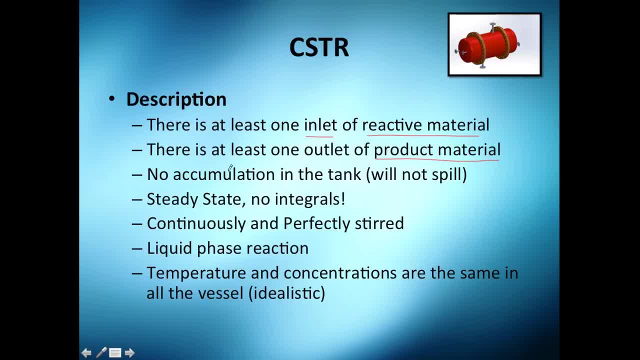 least one outlet of the product. there's no accumulation in the tank, so it will not spill. that's very important. so the volumetric flows are actually the same. you cannot. if you wouldn't have the same volumetric flow, it will either go up or drain. there are no steady states, which implies there's no accumulation. 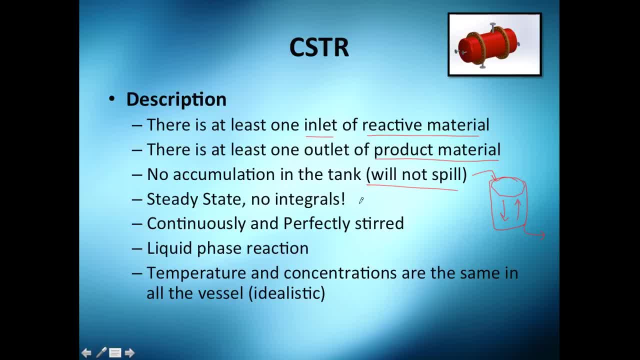 which means there's no derivatives, which means you will not have to do differential equations or integrals. so that's cool. it's continuously and perfectly steered, or agitate with agitation. so you are continually mixing it and it's perfectly mixed. generally it's a liquid phase reaction, so a is. 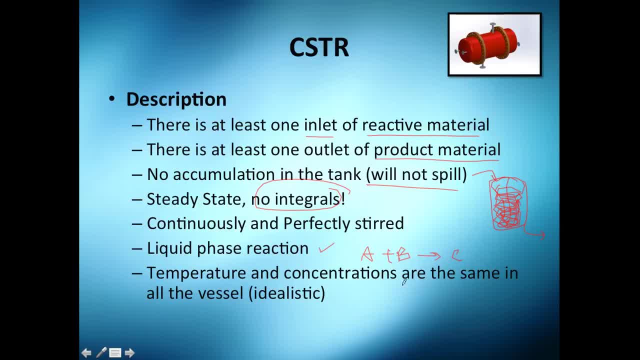 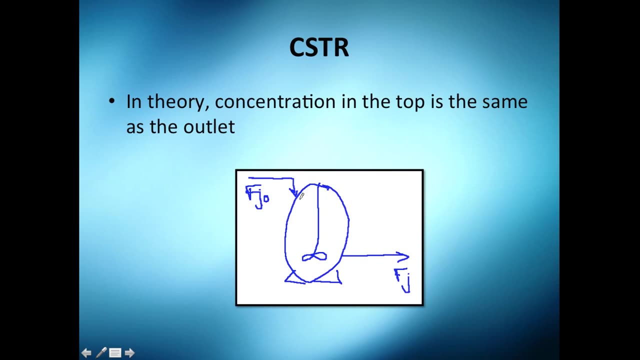 liquid and B is liquid, and you have a liquid product and the temperature and concentrations are the same in all the vessels, which is kind of idealistic, but we need to start with something, so let's start with that. so, in theory, the concentration in the top here is the same in the 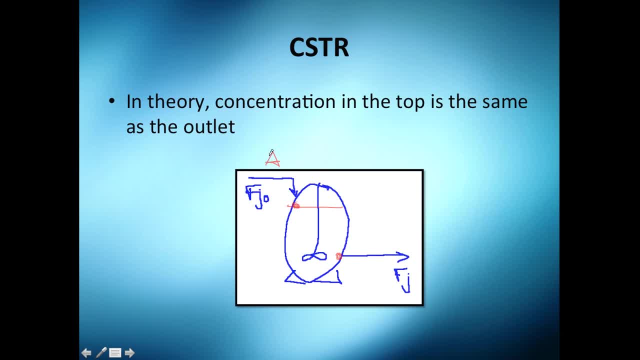 outlet, which is not that real, because if you are feeding A and you are producing B, so you get A turns into B, well, you will have a lot of A here. you will have a gradient now A and B and almost B here. so of course that's not that true. but 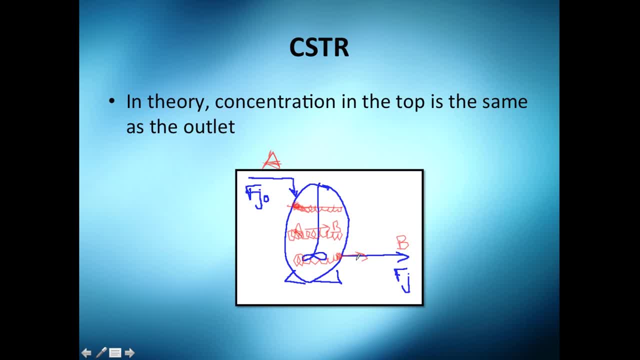 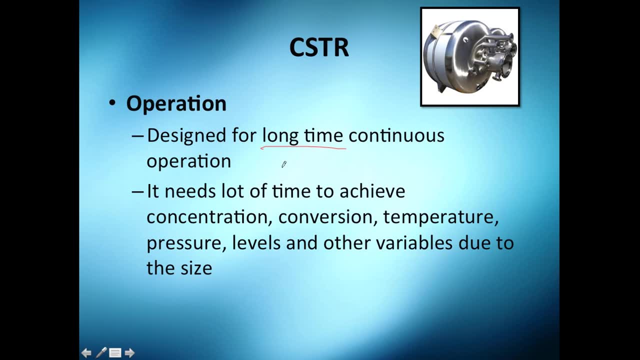 we need to start with something. if you will have a very super agitation system, yeah, it's possible operation. it's designed for long time, continuous operation. I mean you're not going to turn it on one day and turn it off the next day. you want that to operate at least one year, one semester, something. 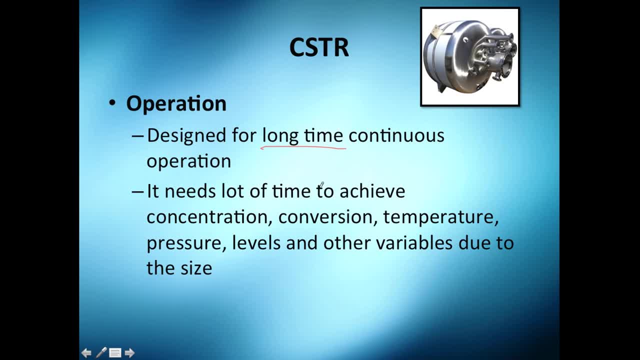 like that. it needs a lot of time to achieve concentrations, and the bigger and complex the reaction, the more time. so you have an idea of how long it's going to take. you know, maybe 10 Celsius and you want to change to 10.5 Celsius. well, you, maybe you think it's going to take minutes, but 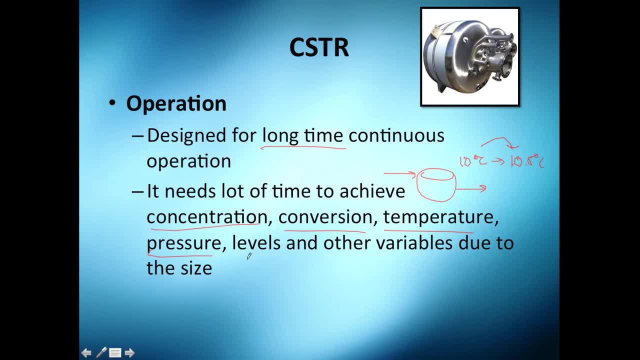 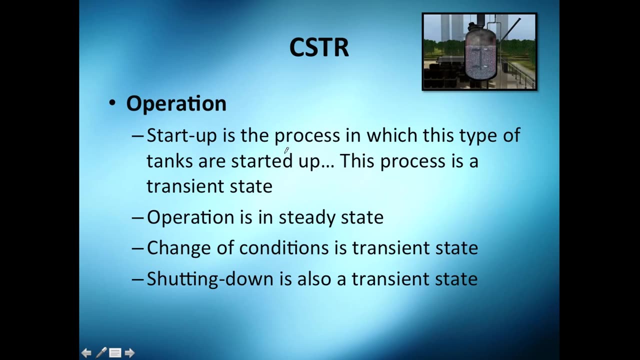 maybe it takes even days. so concentration, conversion, temperatures, pressures, levels and other variables- I don't know- viscosity, densities, all that kind of process variables take time to react or to move. now there is a startup in the process, it's a trenching state. so you're going to, of course, if you have, you have a 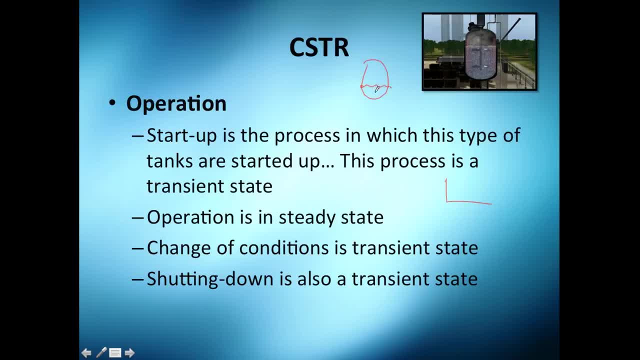 empty CSTR because you're going to start it up. well, you will have to reach a certain level of liquids. that's going to take time, that's why it's a trenching state, also concentrations, also temperatures. you're going to heat. maybe the tank is a 25 Celsius and your operation system is 300, so you're going. 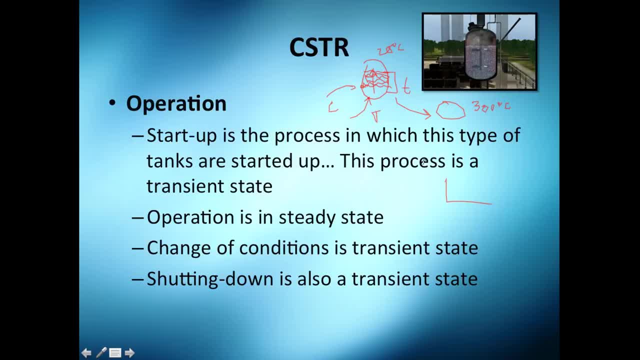 to have also a trenching state in energy. and yes, essentially that's a startup, the operation is in steady state, so we are going to study that part. so I don't know, maybe this part is two days. you operate 300 days. we want to study that in steady state and then I don't know. 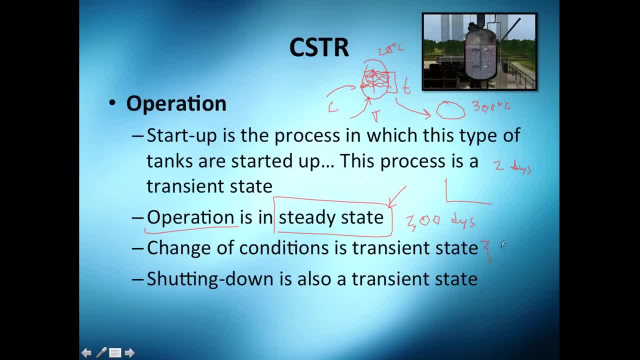 maybe you change the conditions. you will have also trenching state here, but maybe- I don't know- it's one to two days and you're going to operate those conditions- I don't know- 200 days more. so once you're ready, you're ready to go. 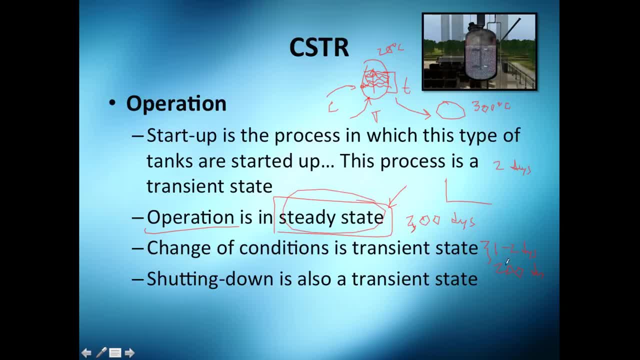 again you have the operations: 200 days, a lot of days. look how the startup or the changing condition or the shutting down are essentially just two to three days in trenching state, but then you operate 200 days, 300 days, all that time. so we are interested more in the operation rather than in the startup, the changing. 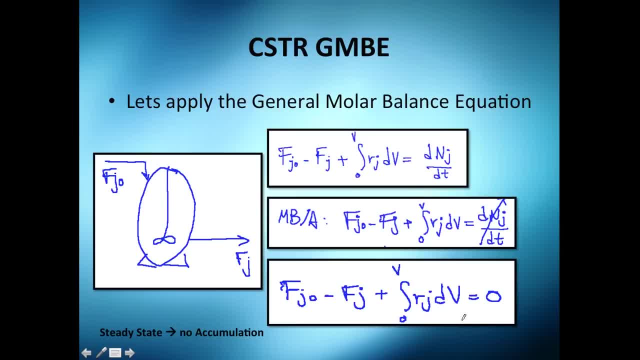 conditions and the shutting down. so, as we've done before with the batch reactor, we're going to do the operations, as you can see here, because it's a set based on. the thing I want to tell you is: I have an inlet, I have an outlet is here and it's. 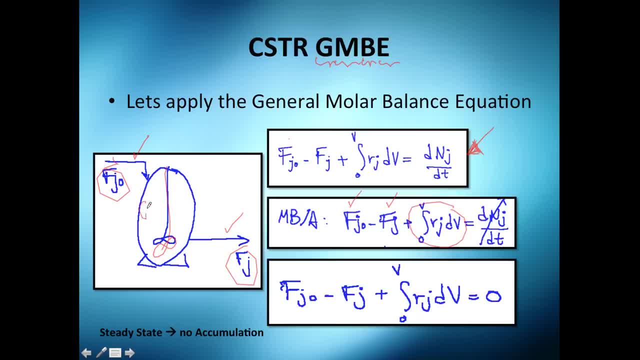 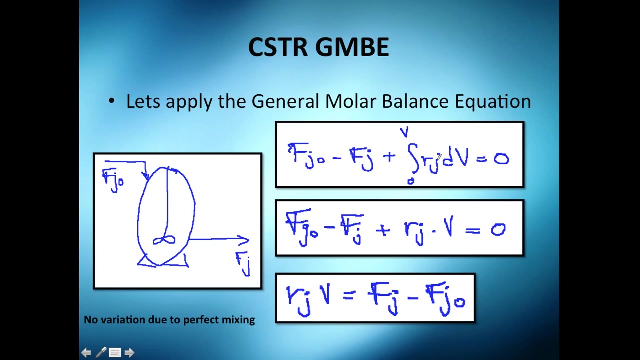 here I got generation because it's a reactor by definition. I'm producing and consuming material and since it's in steady state, conditions do not change in time, moles in A does not change in time. so I got this. inlet outlet plus generation equals zero. now I'm going to take out this rate of reaction out. 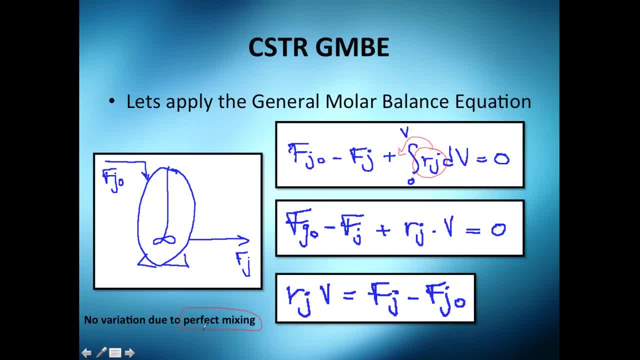 because, since it is perfectly mixed, I can suppose that I can take it out. so the rate of reaction here is the same as rate of reaction here and the rate of reaction here. so I take it out and the derivative. well, the integral of this is one, and you need to evaluate in volume and in zero. this is essentially B minus. 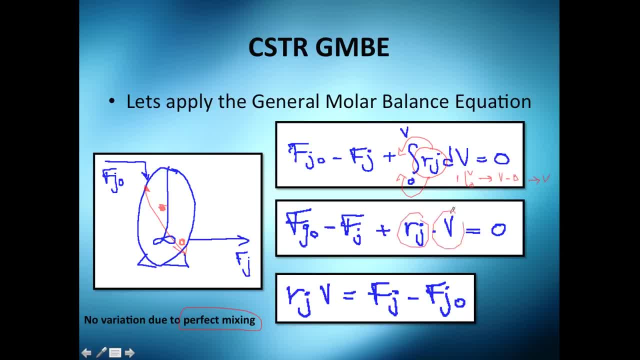 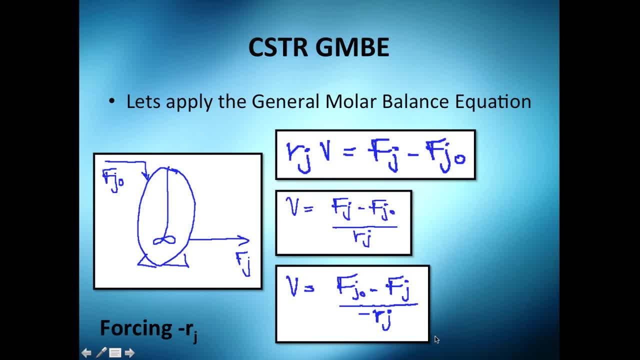 twist them negative and positive, and actually you could let it like that, but I like to leave it in the volume form so I can have a volume directly here. I just change this going deviation and, as I told you before, I'm going to force that negative here because you know rate of reactions. 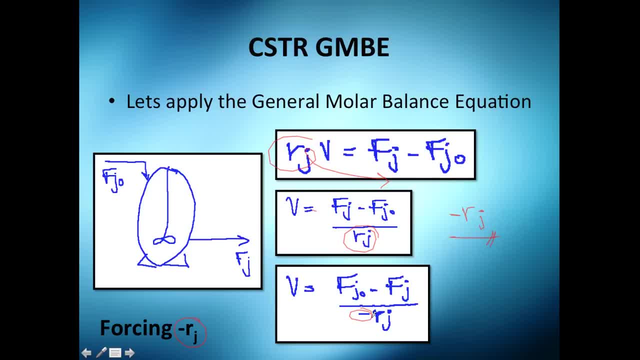 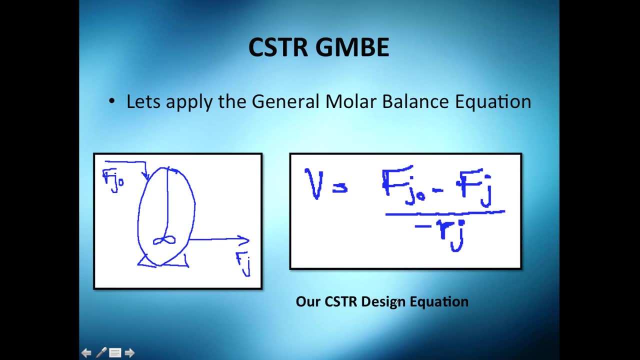 are mainly given as a negative form here. so what do I do? I need to multiply minus here, but also in that. so that's why I twist these guys. so that's my master. continuous to your tank. reaction is so beautiful, so nice. one note I want to add you is that this rate of reaction is. 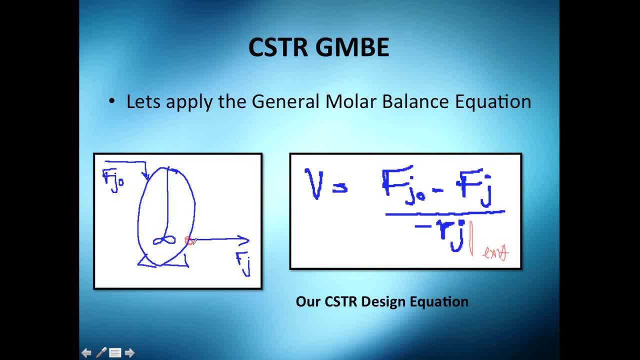 at the exit at this point. okay. so yeah, nice guys, you're done with this CSTR. next we're going to see the plug flow reactor. but this is so simple actually I could give you. I got this inlet flow, it will be. then the outlet flow will be 5. 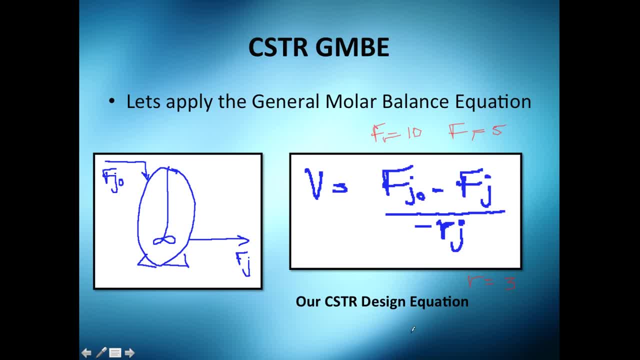 and the rate of reaction is- I don't know- 3. you could calculate right now the volume, which will be 10 minus 5. 5 divided by 3, it's about 1 point, I don't know 6 cubic meters, but that's just a silly and very 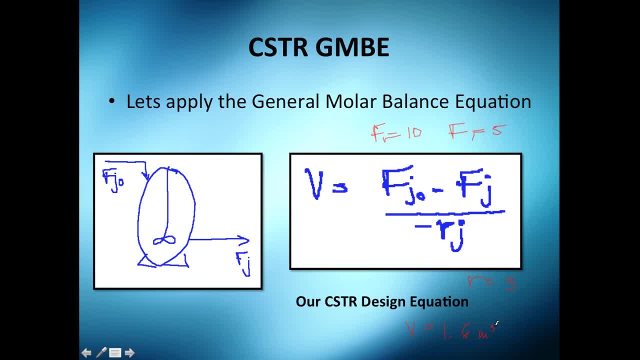 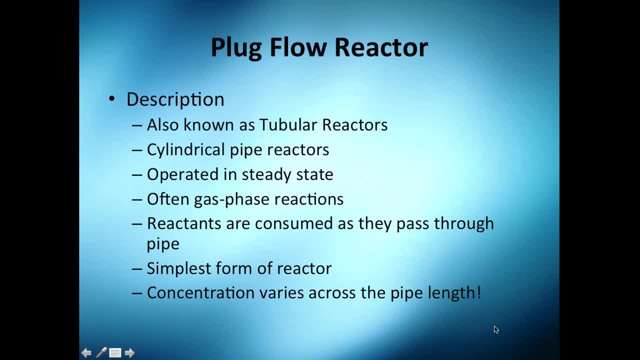 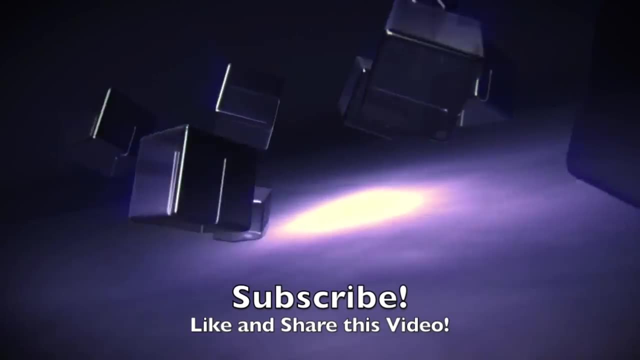 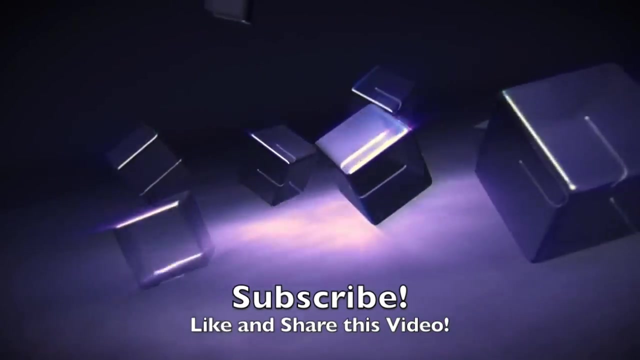 rapid example. we're going to see more examples later. so if you're liking the course, keep in the video or in the playlist. and yeah, let's continue with the plug flow reactor in the next video. what's up guys, it's me chemical engineering guy. so if you like the video, 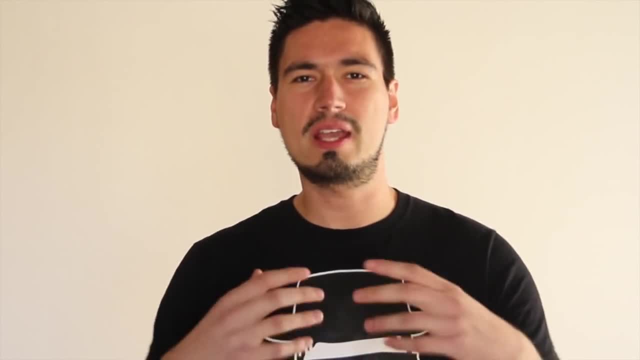 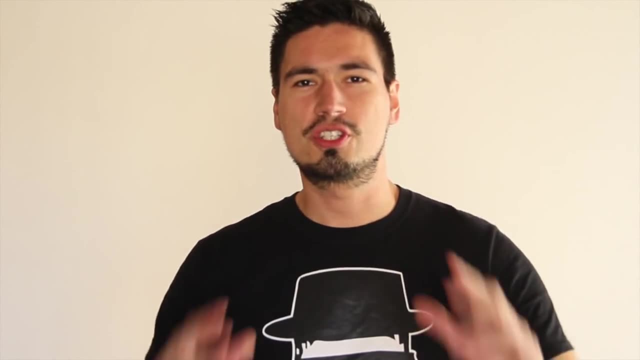 why not push the like button? it really helps me to know if you're liking the videos or if I should be changing something or I should be adding something. taking out content, whatever. also, sharing is caring. so if you got any kind of friends, teachers, colleagues or whatever, 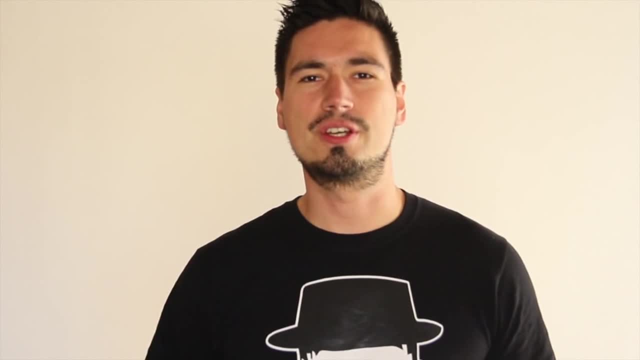 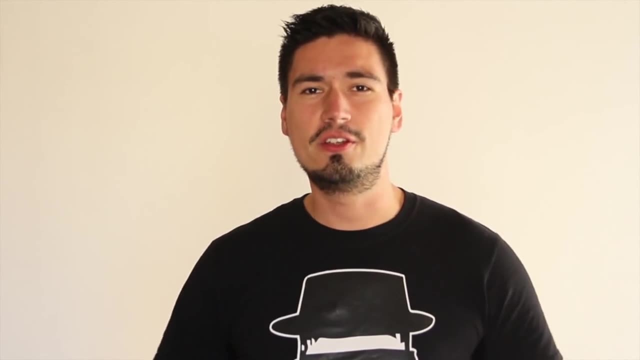 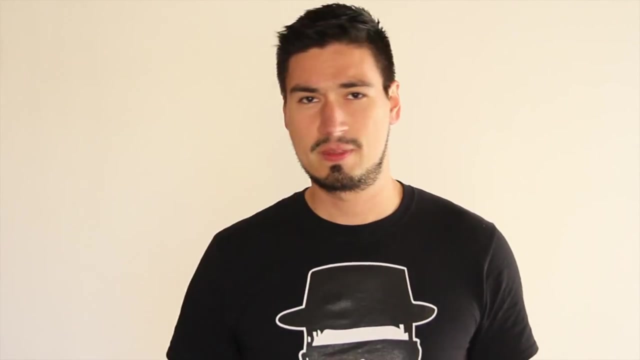 kind of person that might be interested in this type of content. why not share it? sharing helps our community to grow faster- in members and in content. if you want to keep track of my activity- videos, uploads, experiments, plays, whatever content I'm getting YouTube- be sure to click the subscribe button. subscribe to: 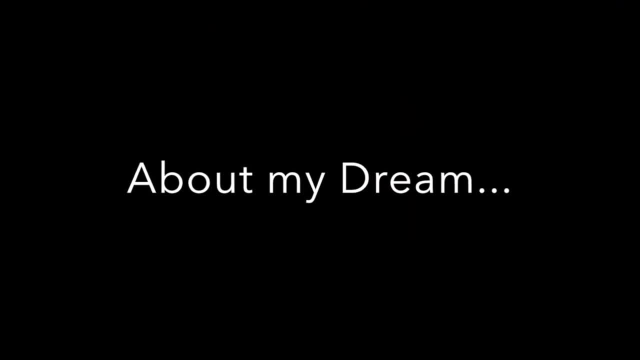 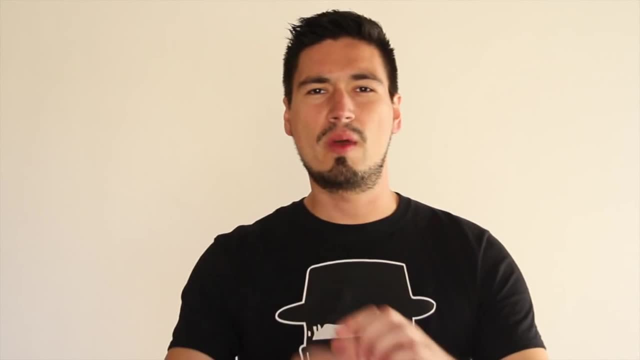 the channel is totally free, guys. my dream is to create an online Academy of chemical engineering where everyone can access it in the future, and I hope you enjoy this video and I'll see you in the next one. bye, bye in the world. imagine a place in which the student, the teacher and the 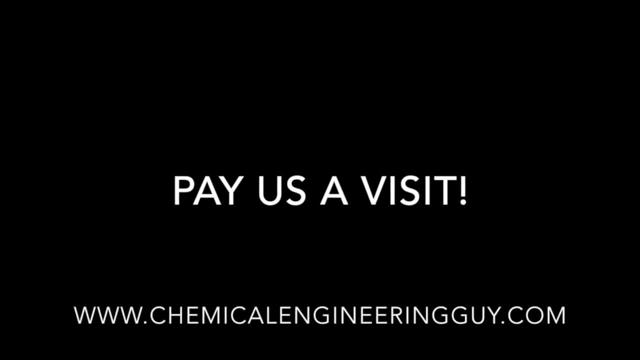 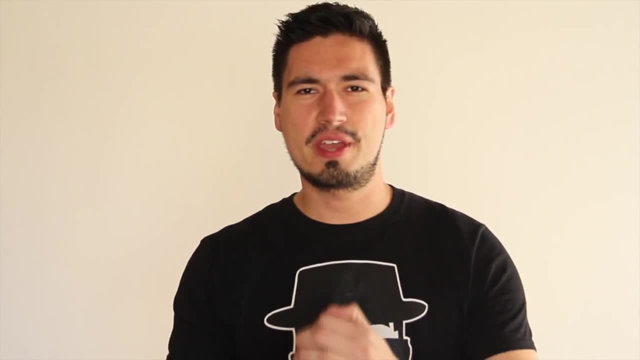 engineer get the best of each other. thank you, thank you. thank you, guys, for the support and the love.